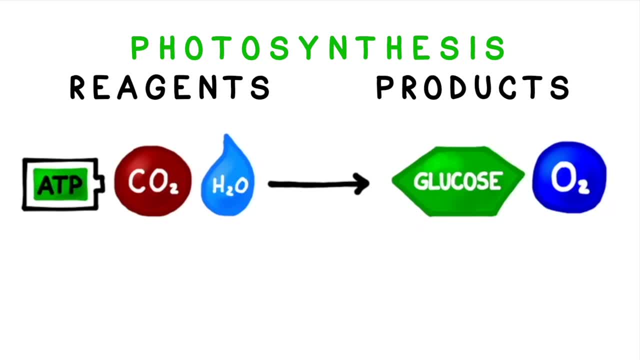 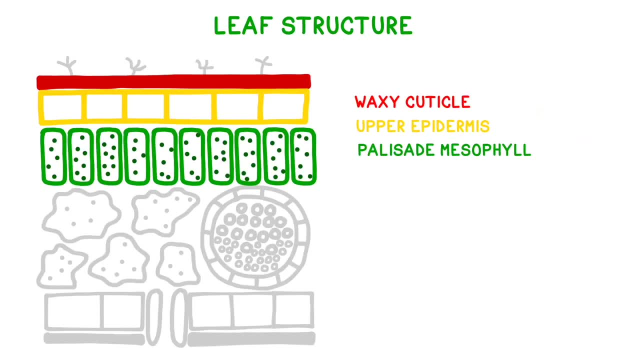 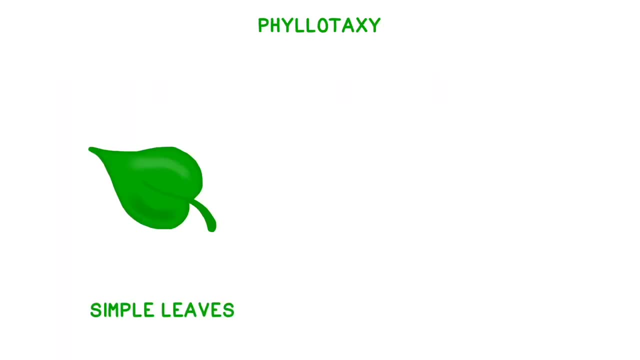 description: During photosynthesis, plants use energy from sunlight to jumpstart the conversion of carbon dioxide and water into glucose and oxygen. As we go through this video, notice which structures are handling each of these reagents and products. There are two major types of leaves: simple. 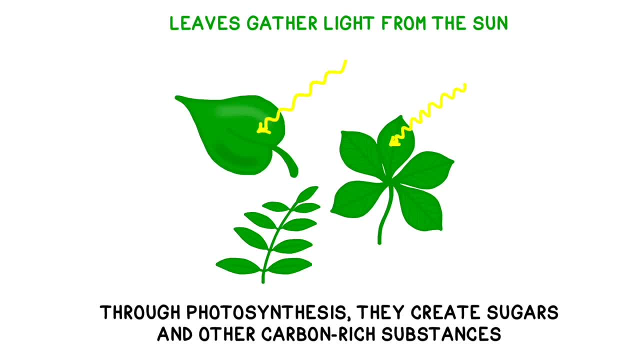 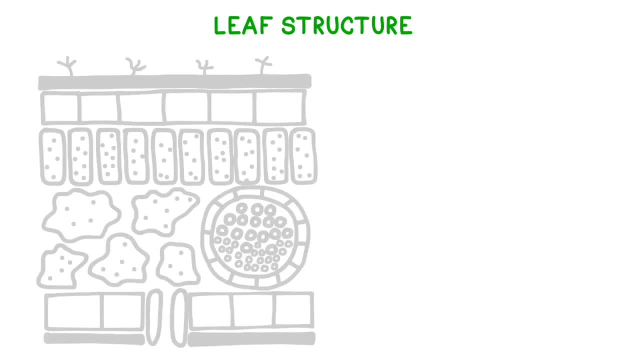 and compound. They both gather light from the sun, so plants can form sugars and other carbon-rich compounds through photosynthesis. The uppermost layer of the leaf is called the waxy cuticle. This is a very thin hydrophobic layer that's on the surface of most leaves. This thin coating helps to reduce water loss. 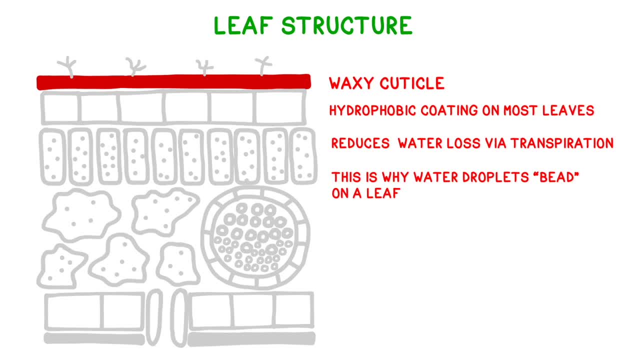 via transpiration, and it's why water will be bead on the surface of leaves rather than soaking in. The first true layer of cells is called the upper epidermis. These cells are tightly packed in order to help prevent water loss In very hot or very cold climates. sometimes this 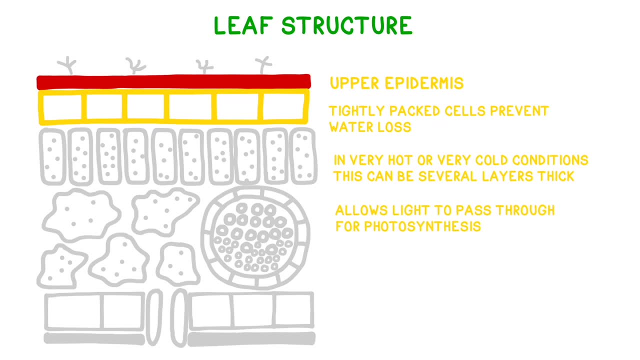 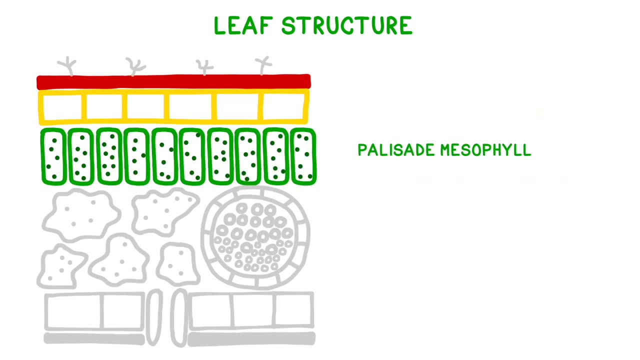 layer can be several layers of cells thick. Because the upper epidermis is translucent, it allows light to pass through for photosynthesis. The next layer is called the palisade mesophyll, sometimes called the palisade parenchyma Palisade. 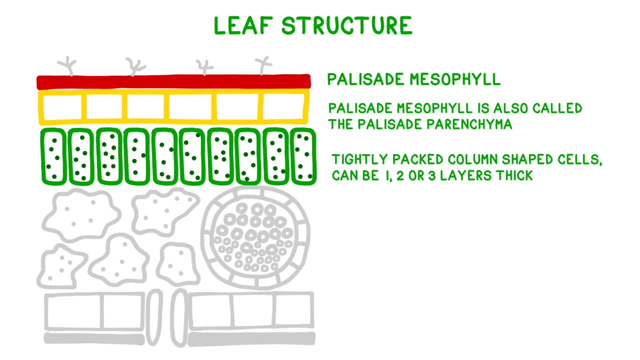 mesophyll cells are tightly packed together and column-shaped Because this is the major site of photosynthesis. they are full of chloroplasts and there are often several layers of this type of cell. Photons of light will shine down through the waxy cuticle and upper epidermis. 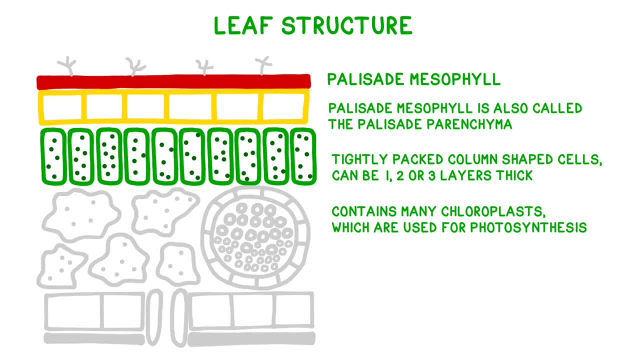 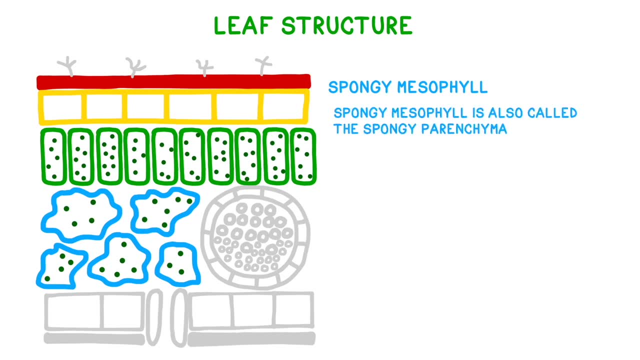 in order to strike the chloroplasts that are located within this layer of tissue Beneath the palisade mesophyll is the spongy mesophyll. The spongy mesophyll can also be called the spongy parenchyma. These cells are more irregularly shaped, so they are more likely to form a 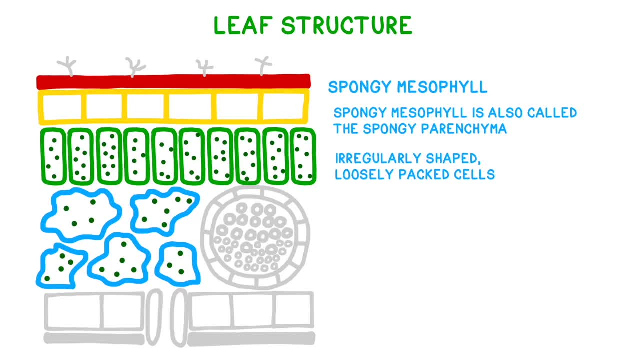 shape relative to the palisade mesophyll, but they do contain a few chloroplasts, so some photosynthesis does take place here. The space in between these cells is called the intercellular space, and this allows for gas exchange in and out of the leaf. 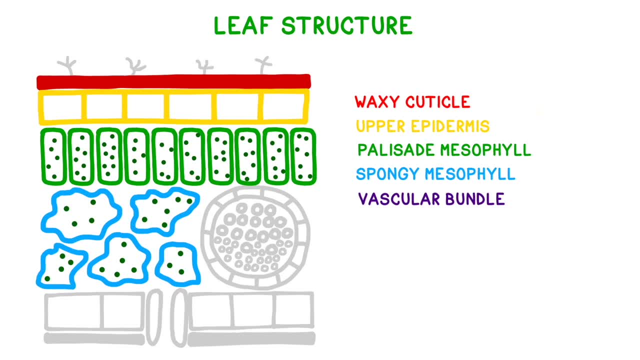 The next structure, called the vascular bundle, consists of several different types of tissues. The first tissue is known as xylem. Xylem is a vascular tubule within the plant and its flow runs upwards. It's used to transport water from the roots to the rest of the plant. 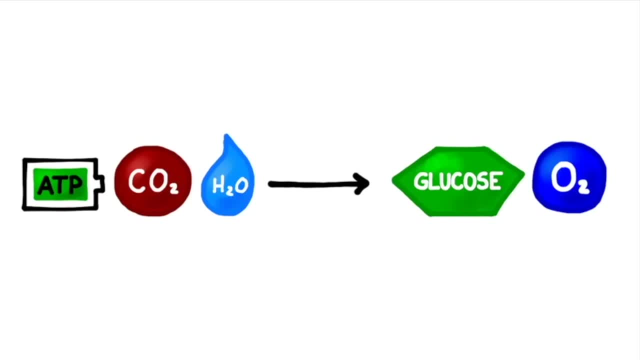 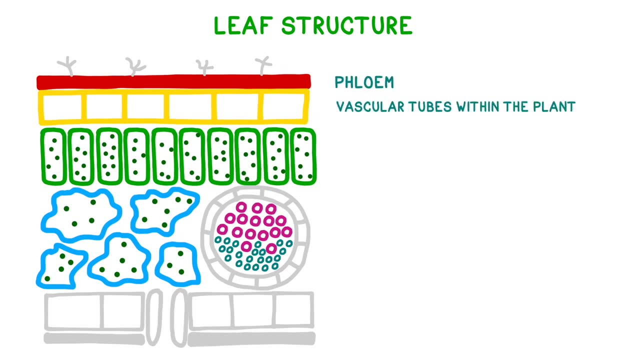 wherever it's needed. Remember that water is a necessary reagent of photosynthesis. Phloem is xylem's counterpart. These are also vascular tubules within the plant, but its flow runs both up and down. It's used to transport the products of photosynthesis. 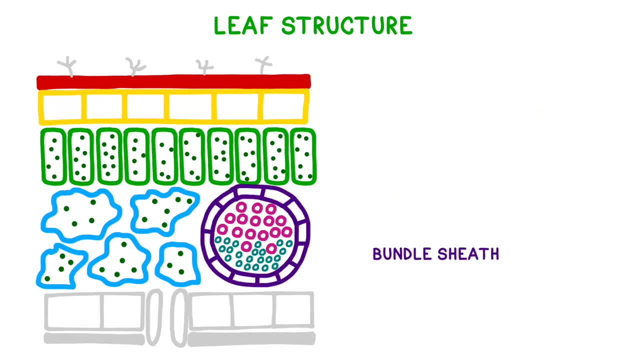 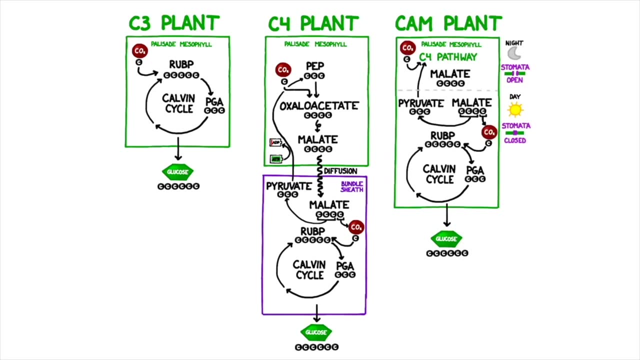 from the leaves to the rest of the plant. Surrounding the xylem and phloem is a network of tightly packed cells called the bundle sheath cells. In some plants, bundle sheath cells allow for a specialized version of photosynthesis that allows plants to survive in arid or dry environments. We can see the role that bundle 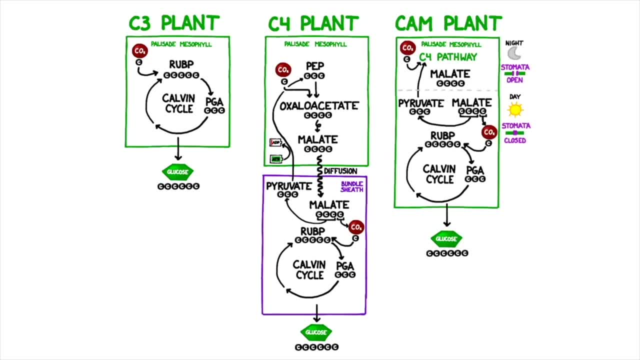 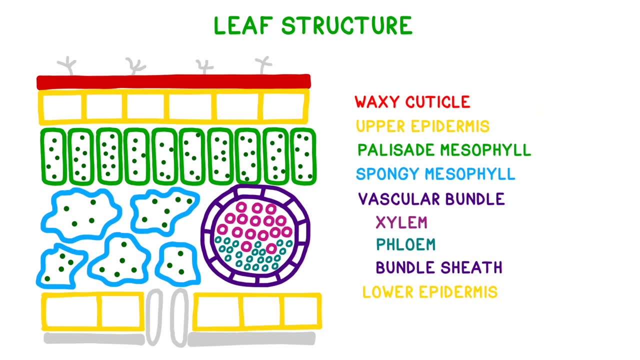 sheath cells play in this diagram of the C4 photosynthesis pathway. The lower surface of the leaf also contains a layer of epidermal cells called the lower epidermis. This is also meant to prevent water loss. Within the lower epidermis we can sometimes see a small opening called a stoma. This series 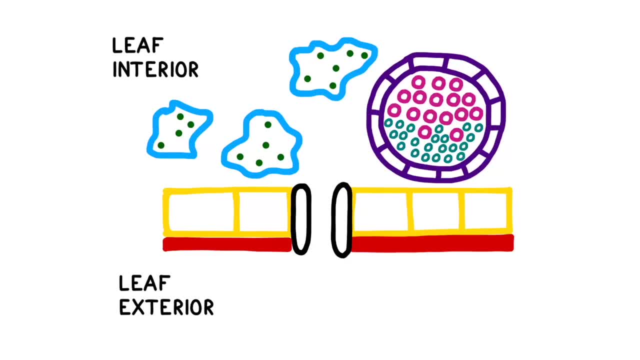 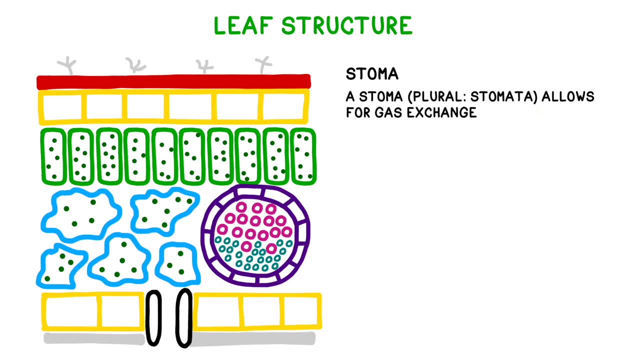 of openings allows for gas exchange in and out of the leaf. Ideally, carbon dioxide will diffuse in and oxygen will diffuse out. Each stoma has two guard cells, one on either side, which can open and close in response to the environment. If it's very hot, the plant will likely keep its stomata closed. 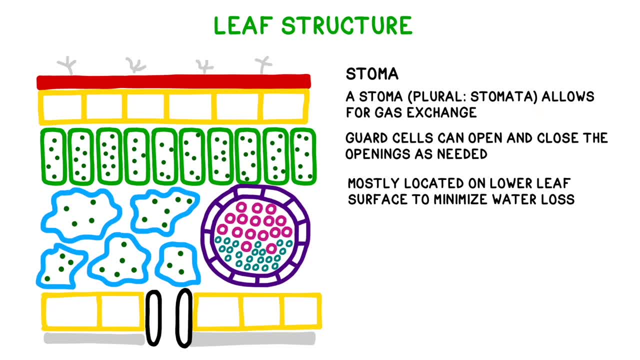 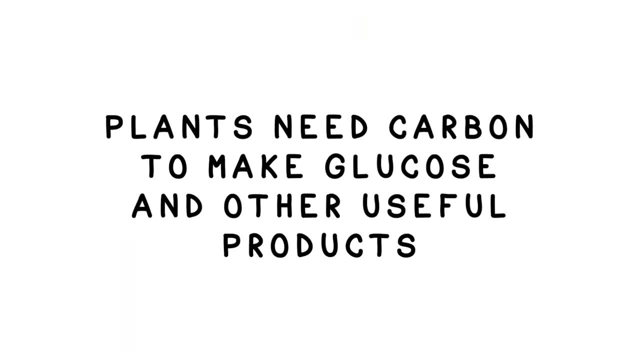 in order to minimize water loss via transpiration, Most of the stomata are located on the lower surface of the leaf rather than the upper. In order to make glucose, as well as a number of other plant products, plants need carbon. To get the carbon out of the leaf, the plant needs to use carbon dioxide- Carbon dioxide. 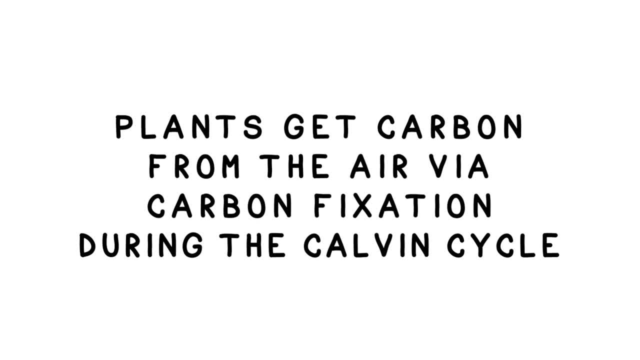 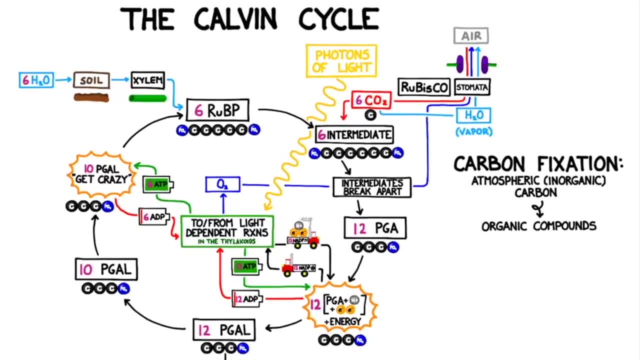 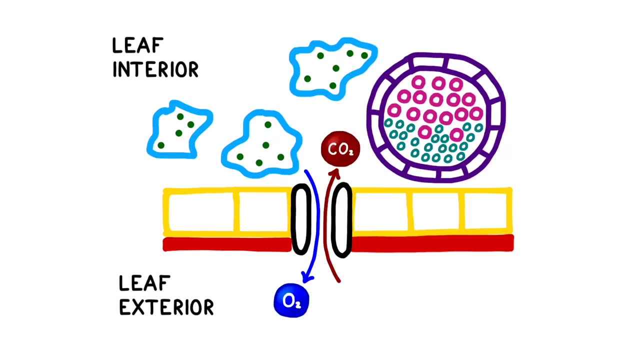 is a process called carbon fixation. To get the carbon that they need, plants have to extract it from the atmosphere in a process called carbon fixation. During photosynthesis, they take atmospheric carbon from carbon dioxide and convert it into organic carbon contained within molecules like glucose. 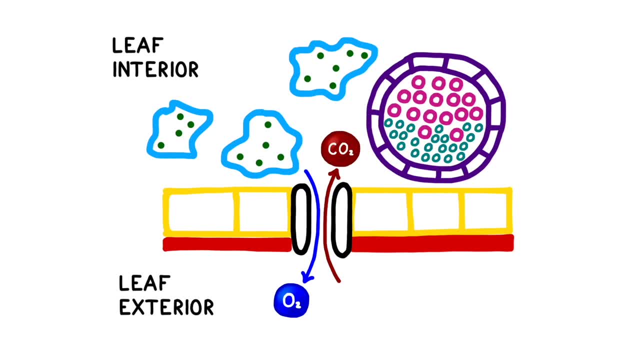 For plants that live in a hot environment, this is a delicate balancing act. They need to keep their stomata open enough of the time to get carbon dioxide in, but not so often that they allow themselves to dry out. C4 and CAM. plants which live in dry environments have a number of different ways of getting. 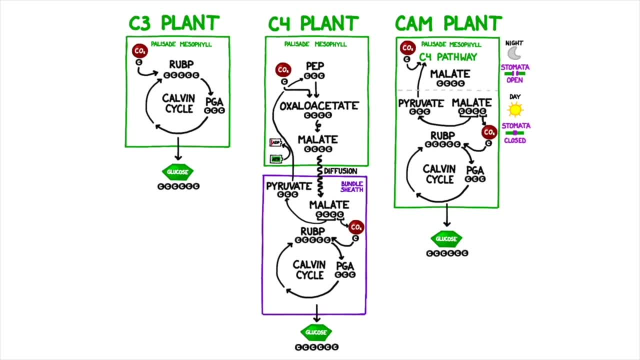 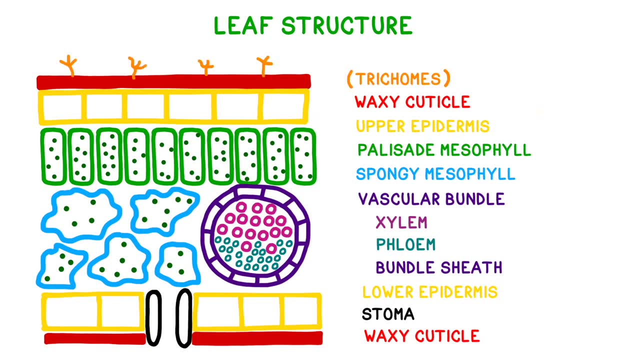 around this problem, including using a modified form of photosynthesis. The lower portion of the leaf usually also has a waxy cuticle, much like the upper portion. Many leaves have additional structures on their surface, known as trichomes. These can perform a variety.